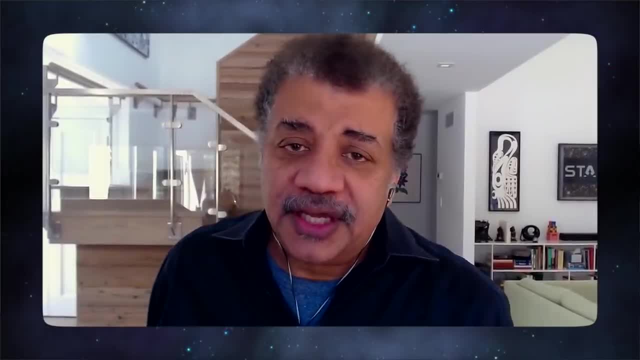 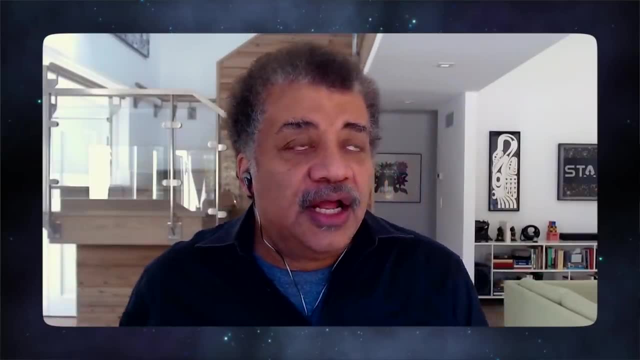 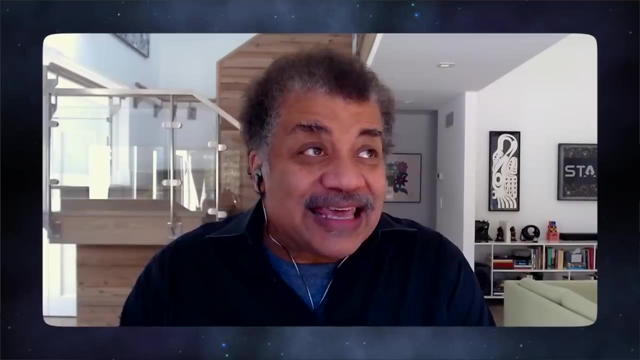 you go to a fast food restaurant and then I ordered French fries, Okay, That's kind of cool. And then, you know, for turkey dinner there's mashed potatoes, right. And then in the breakfast, brunch, you know diner- you can get hash browns. Yes, Okay, I think I was 11, maybe 10. 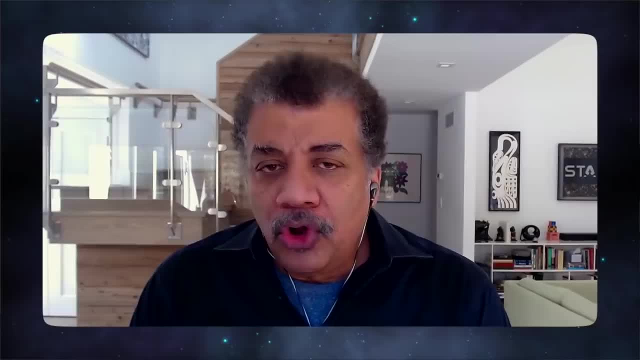 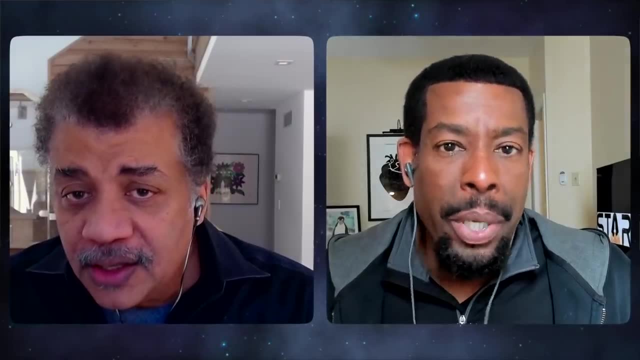 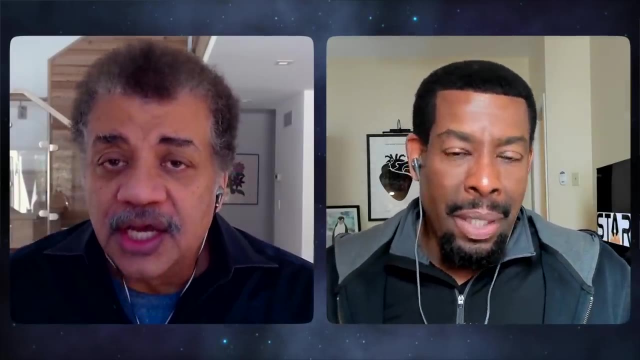 before I figured out that all of those were the same food, Right? Well, I mean, it's nothing to think about when you're 11 or 12.. It's just food. It's just food And it's it's delicious. And only one of them- two of them- have the word potato in it. That's a mashed. 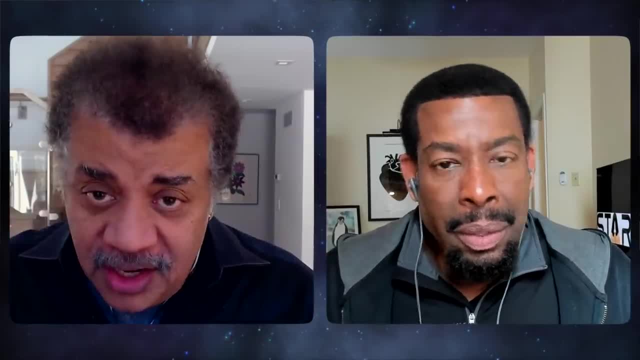 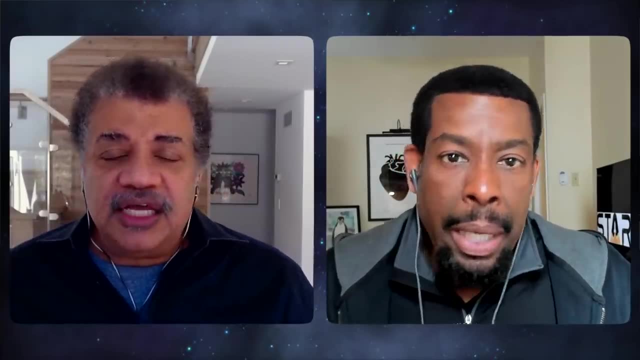 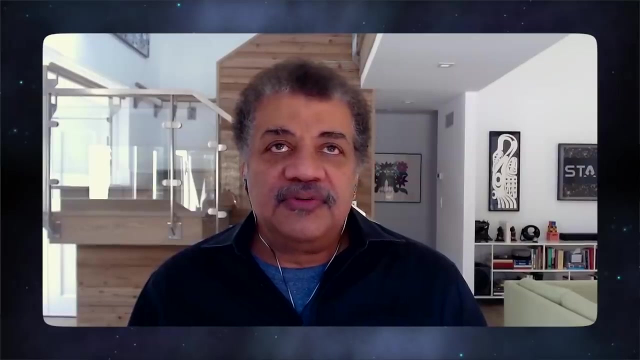 potatoes and potato chips, but they are completely different from each other. And French fries that no one says potato. and hash browns: they don't say potato. So I grew up on freedom fries. So they don't even know what freedom fries Okay. So so it was a. it was a revelatory moment for 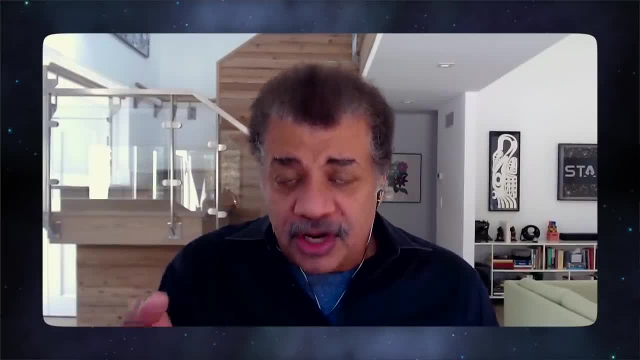 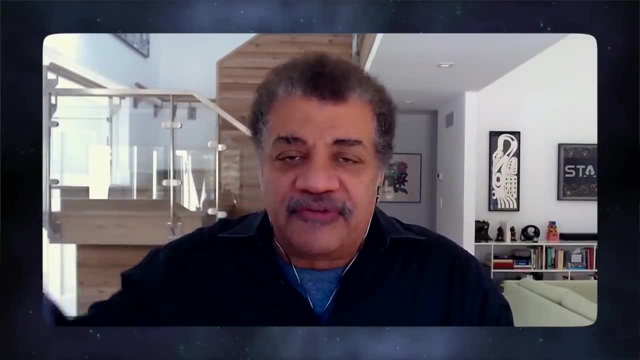 me to realize that one food could be made so different And so So interestingly different to have its its own place within our culinary offerings. Each one of those could do that Right. Oh, another one I liked were the potato sticks. Do you remember those? 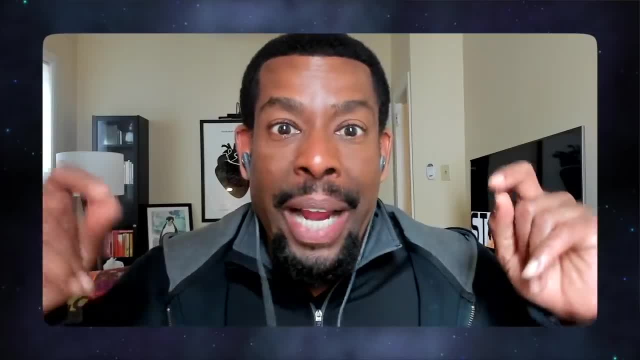 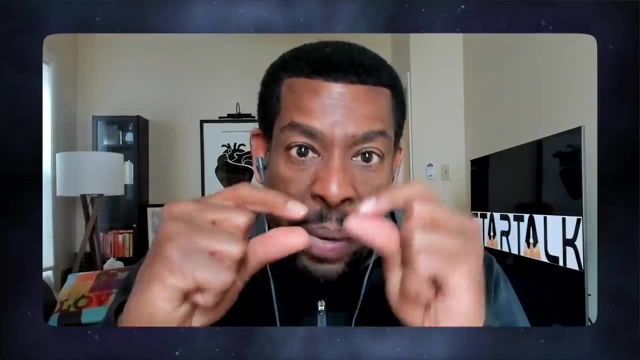 Oh God, Yes, man, Do you remember the potato sticks that, um, uh? oh well, yeah, they're, they're the same thing, Nevermind. So they had. they were like French fries, They had the big. 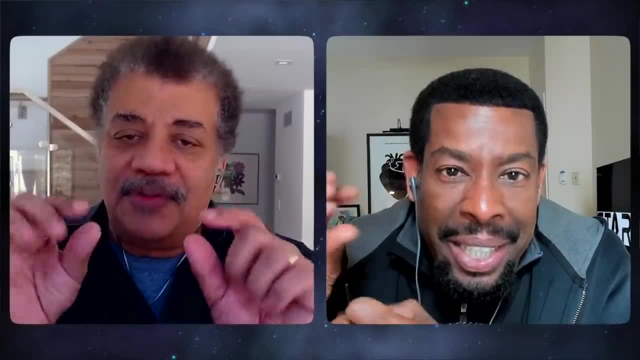 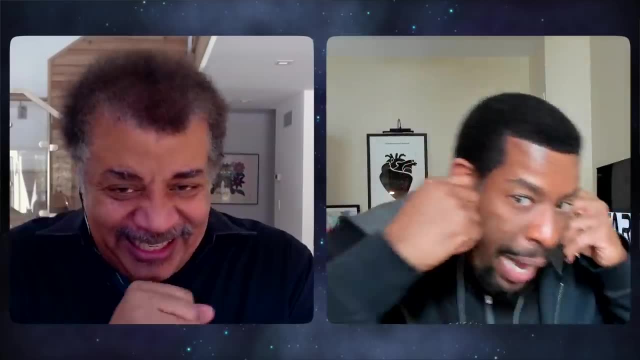 potato sticks. and then they had the tiny little matchsticks: potato sticks, The matchstick, Those were the best, Cause it was like a lot of salt, Okay. So the point is: okay, I am starving, I'll be back, I'll be right back. So they were all different, yet They were the same, Right. 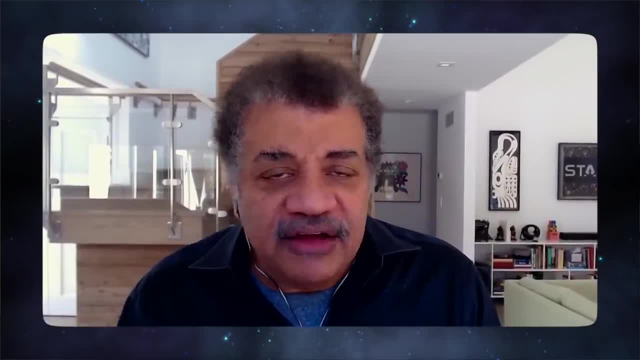 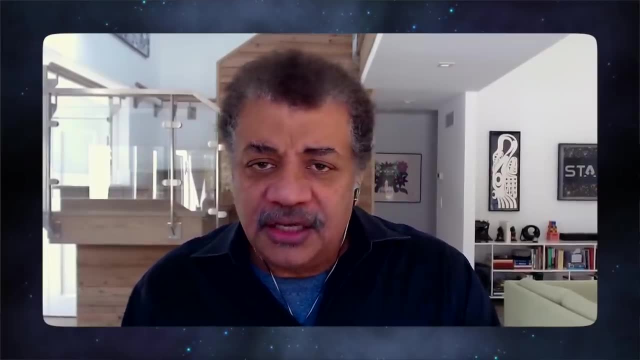 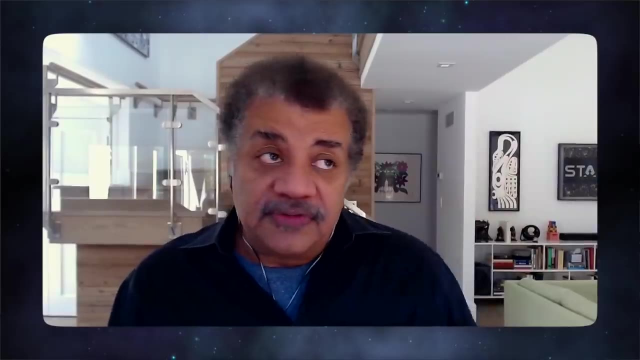 Right, And so too was my revelation of middle school. early middle school, It was probably probably sixth grade now. where cause I was an early geek, but realizing that, okay, you've heard of these things called microwaves, You've heard of radio waves. 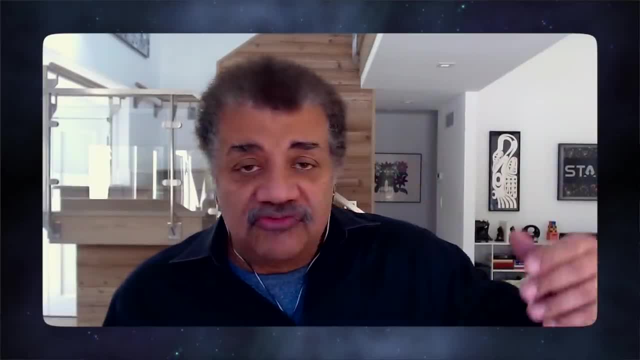 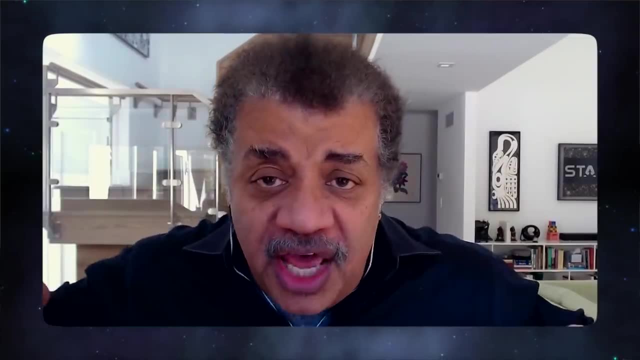 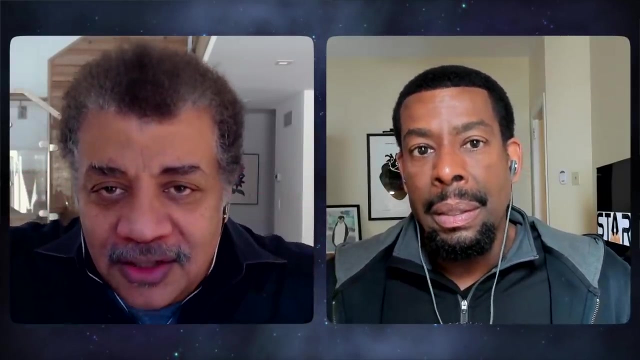 You've heard of uh, infrared ultraviolet. You've seen rainbows, visible light. you've heard of x-rays, You've heard of gamma rays. It's all the same thing, Right, It is. it is just different ways of preparing your light. Okay, To use my potato analogy, 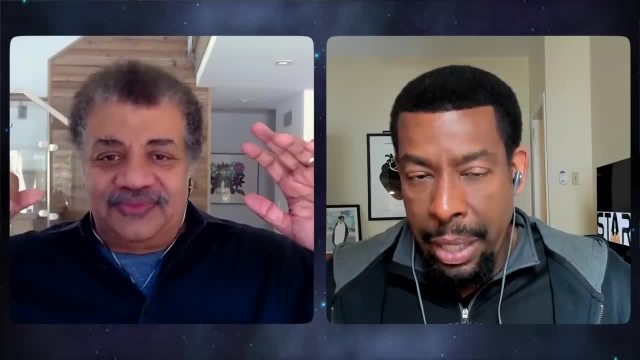 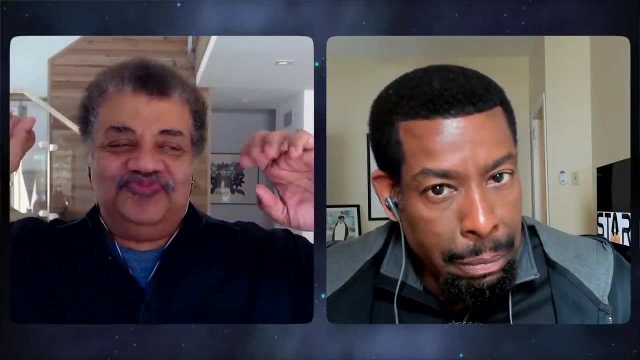 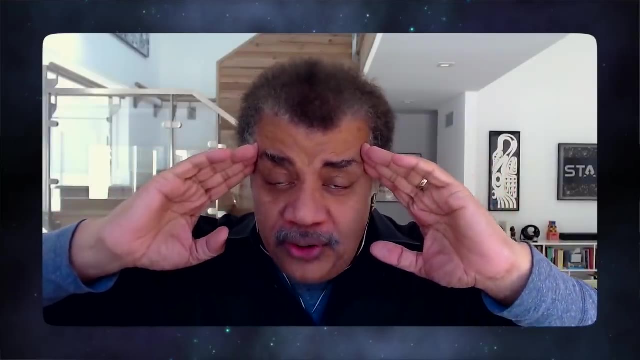 And so you're basically 11 years old and you're making this discovery for yourself, After I realized about the potatoes- Yes, Okay, Cause I was 37. So so I said: my gosh, it's all light. It all travels at the speed of light, And this word light. 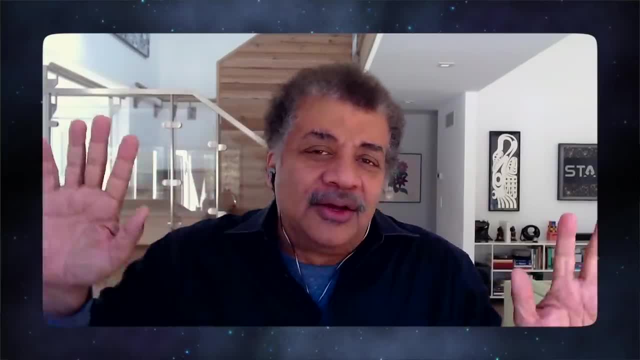 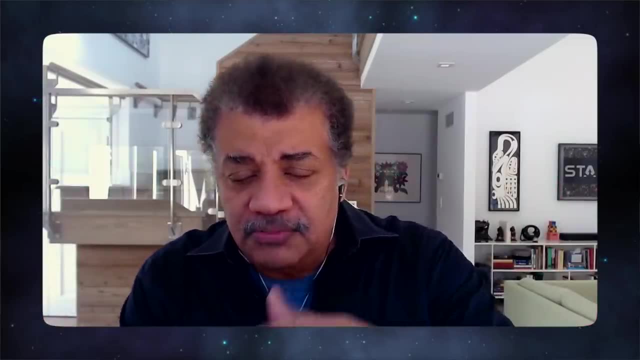 where you're talking about what the human retina can see. that's very limiting, for if you want to talk about the universe because, so what's the our favorite light colors? red, orange, yellow, green, blue, violet- Okay, Continue there And you go to the other side of. 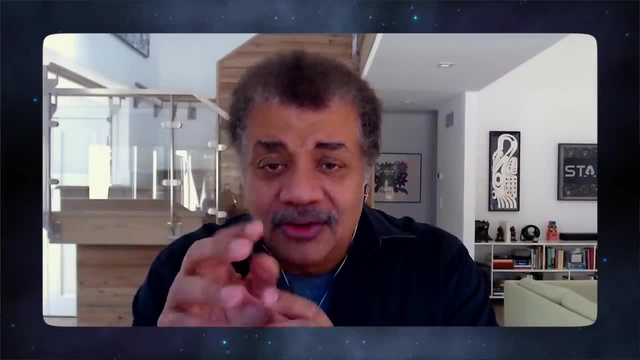 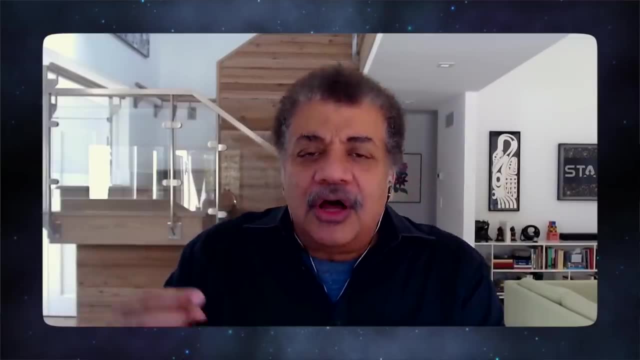 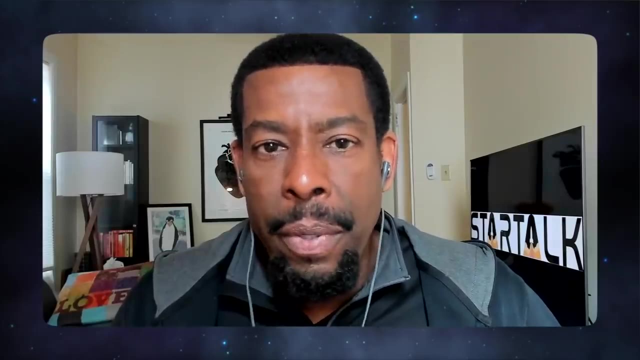 violet, You get ultraviolet. You go beyond violet. That's how it got its name. It's beyond violet And we abbreviate it UV. but I like flesh and ultraviolet. Give me, give me all the syllables that it's got, Okay, And this is the sounds. far more harmful. In fact, it is because 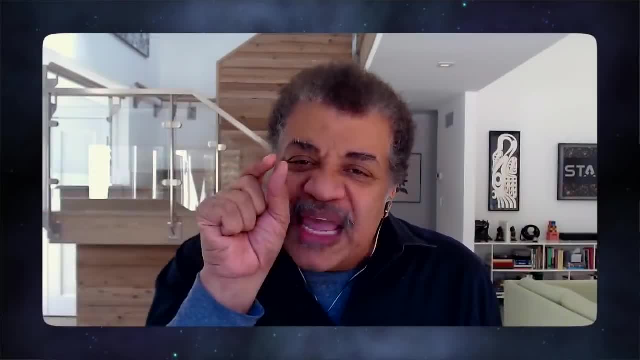 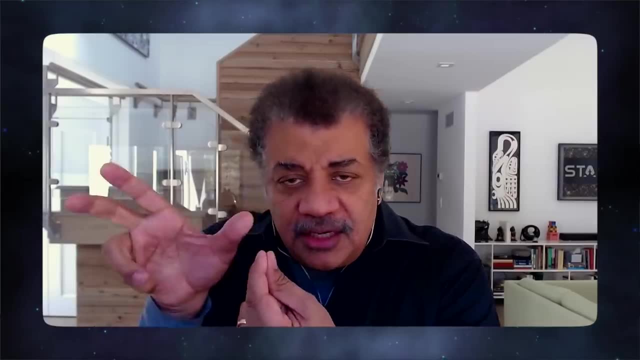 this in this direction: we are reducing the wavelength of light that's coming to us, And when you reduce the wavelength of light, more energy is packed into one pulse of that light, And so the energy goes up. Well, okay, Okay. 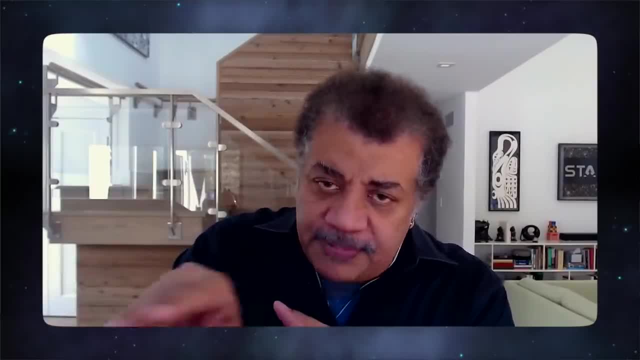 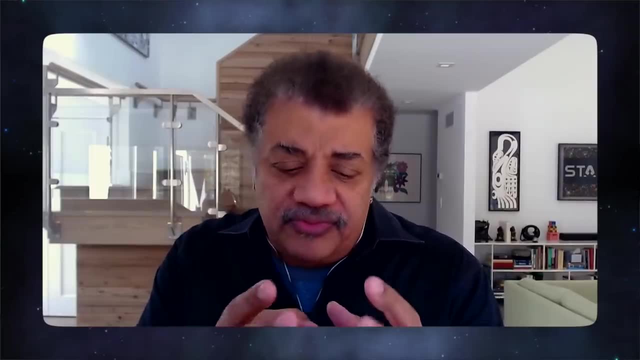 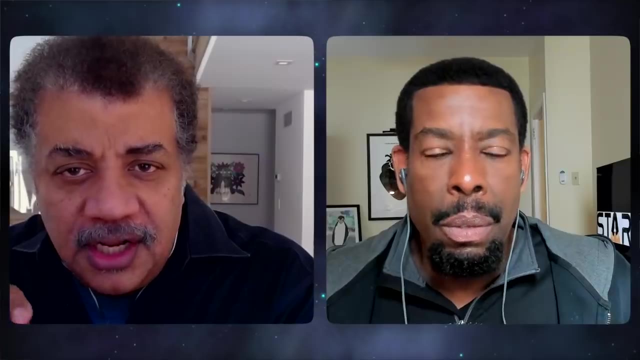 So the higher the frequency- it's how many crests go by per second- The higher is the energy of that light. So the red, orange, yellow, green, blue, violet is all sort of pretty harmless You get into ultraviolet light. It has enough energy to break apart biological molecules And this will 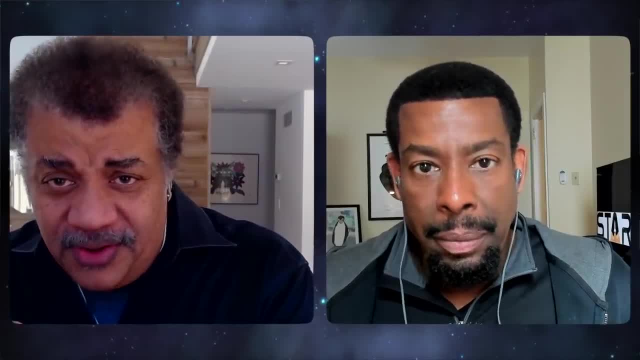 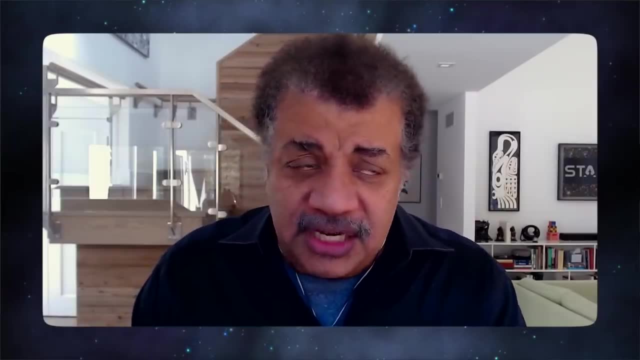 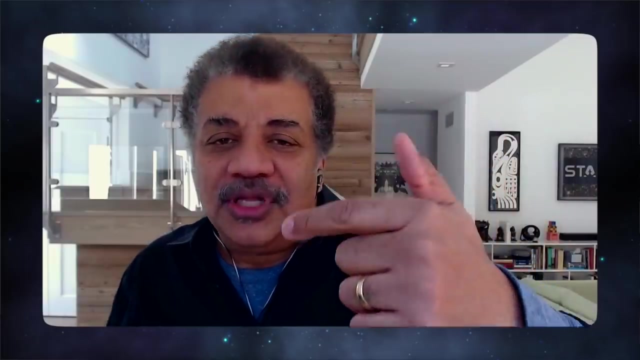 give you skin sunburn and skin cancer, Right, Okay. So I heard a DJ talk about when he just learned that the temperature on Venus was 900 degrees. He said, well, you better bring sunblock a million for that. So he's wrong. He's thinking that you- you you're protecting from the heat. 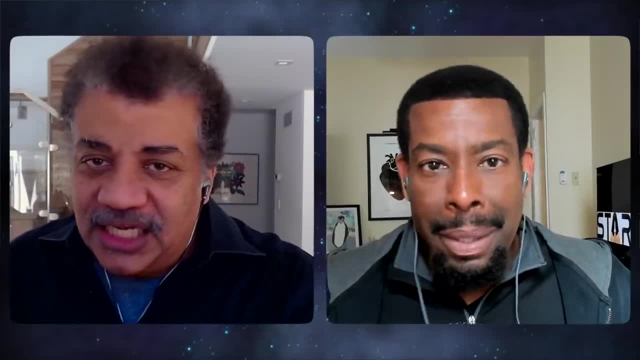 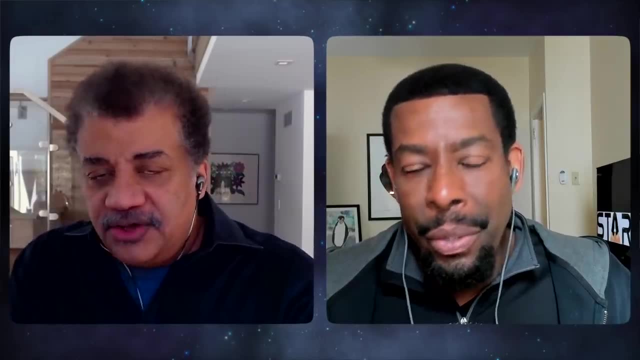 That you can block that, Right. No right, You're not blocking heat, Right? The point of the sunblock is to block just the UV, Just the UV, Okay, Right. So So you still, you still get dark and 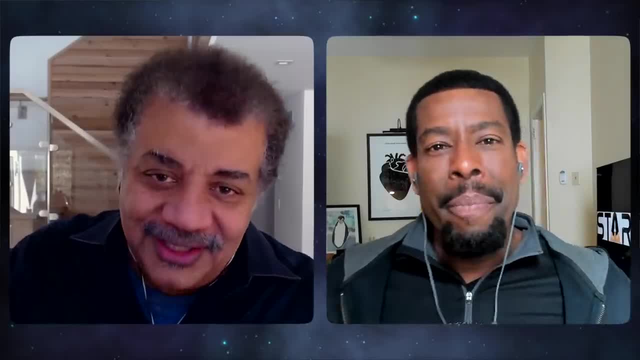 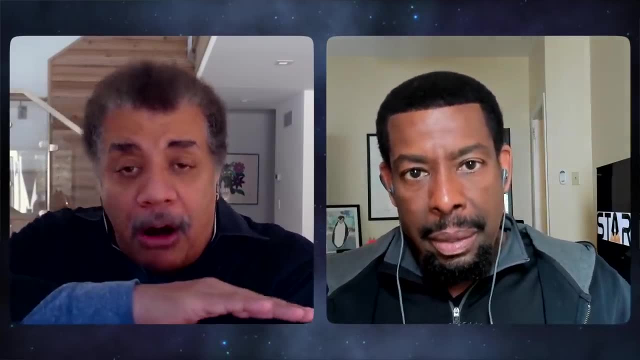 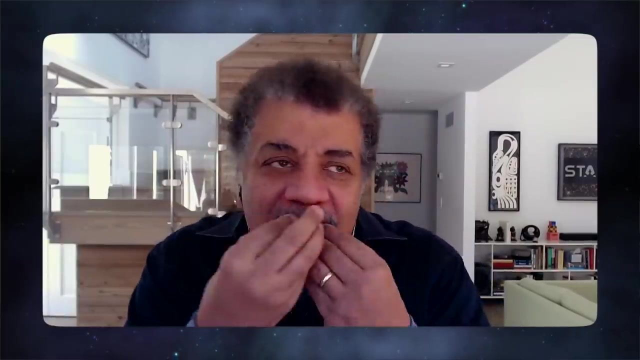 crispy, no matter what you want to do, Yeah, You'll get toasted, You're toasted, No matter what, No matter what. So then you go beyond the ultraviolet, and that's when you get the x-rays. Right. It is continuous with the ultraviolet, Right? We put a line there just because of our convenience. 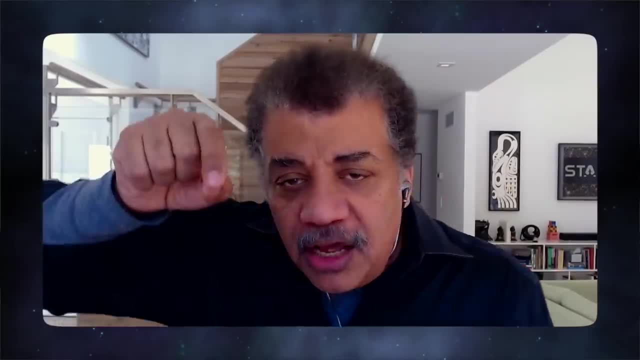 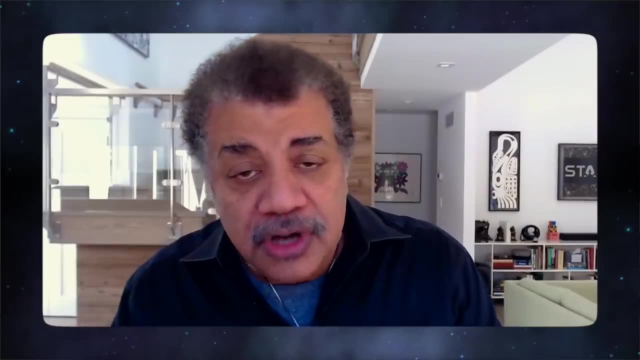 of words and machines built on it. But. but ultraviolet smoothly transitions to x-rays. Interesting, Okay. And and you know, x-rays are bad for you, because when you go in the x-ray room, what does the x-ray tech do? 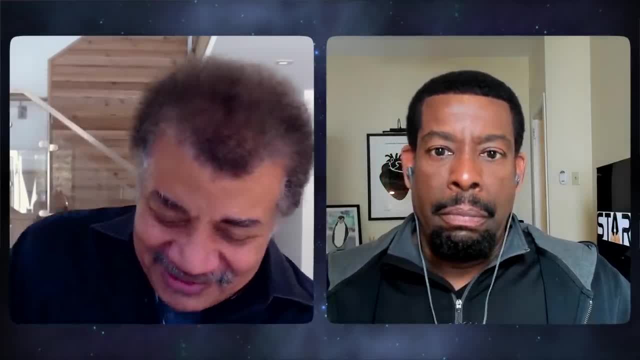 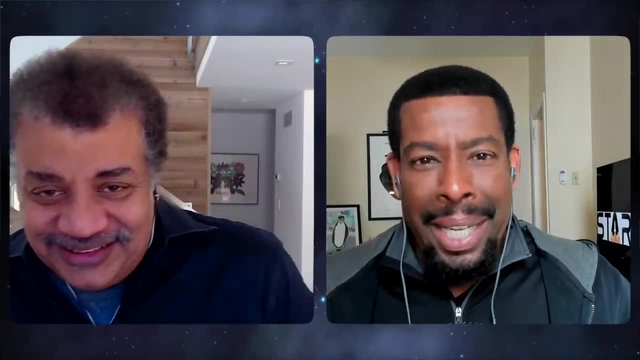 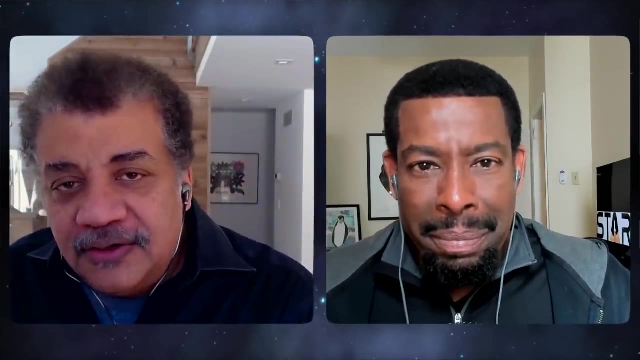 Um, they go to a bomb shelter. They leave the room, They say: are you okay, Are you comfortable? Yeah, Okay, Boom Door closes, Exactly, And they look through a LED, LED glass, and then they okay. So, uh, so x-rays can actually. 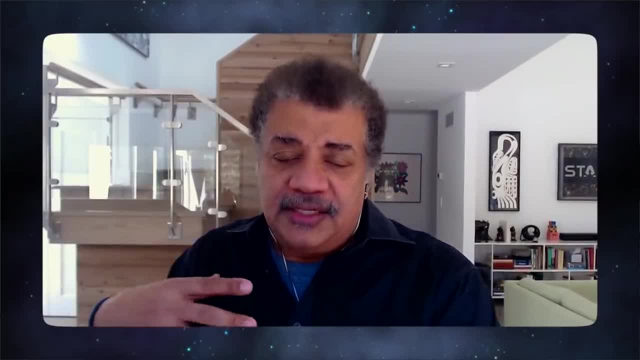 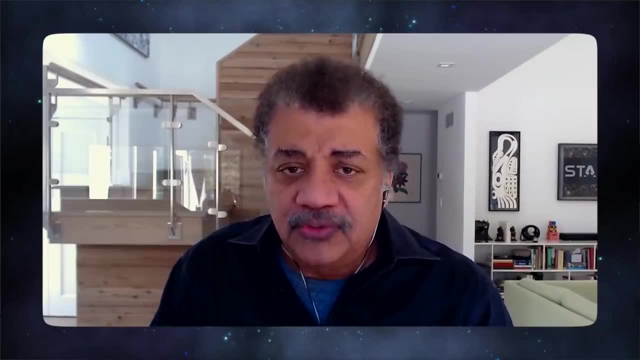 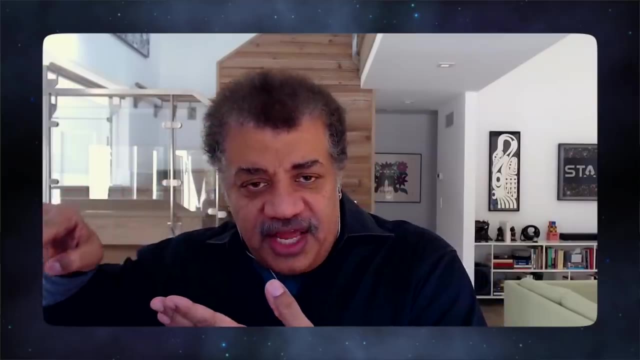 penetrate your skin, unlike ultraviolet, And in doing so, uh, it can actually harm your organs. All right, And so you get organ failure from it And organ cancers are triggered by this. now it's once again. it's a continuum of a change of wavelength of light, and then you get to beyond. 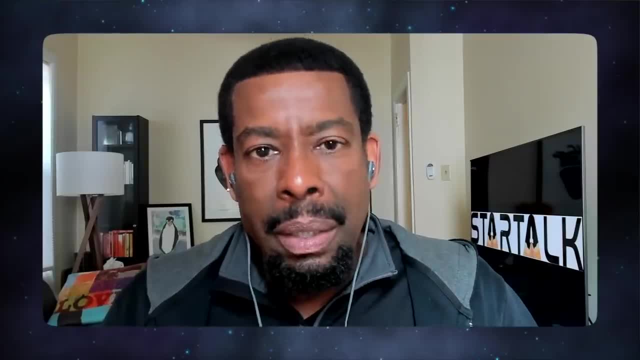 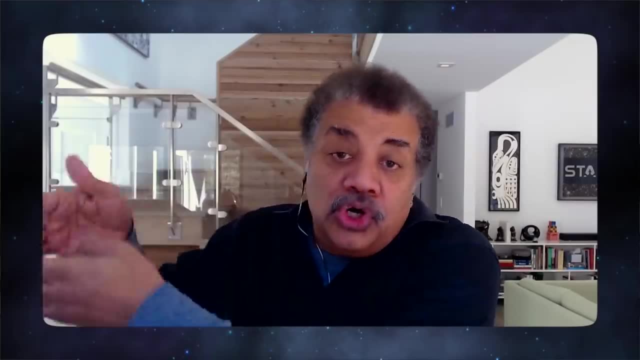 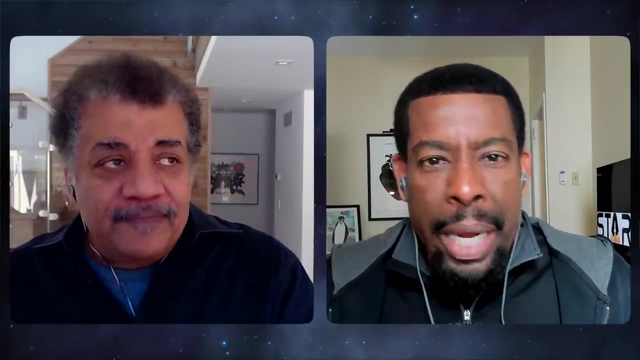 x-rays, you get to gamma rays, right, and, by the way, gamma rays just keep getting higher and higher energetic. but we don't have more words for it, right? it's just the last word we've got, but you could have divided that up even more. we just don't, okay, and so gamma rays get omega rays, or something. 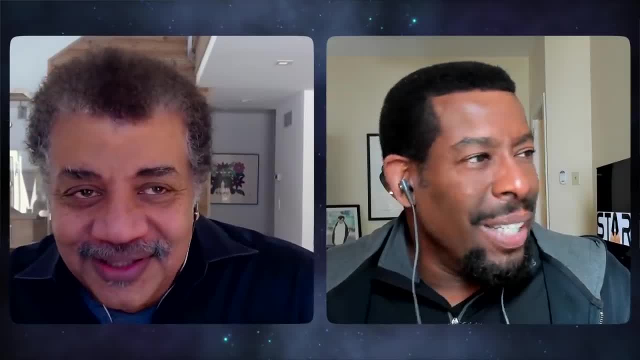 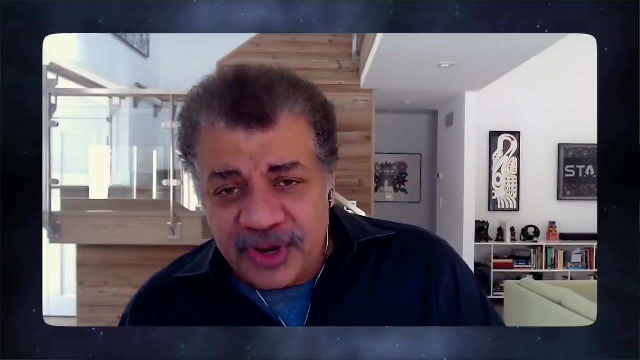 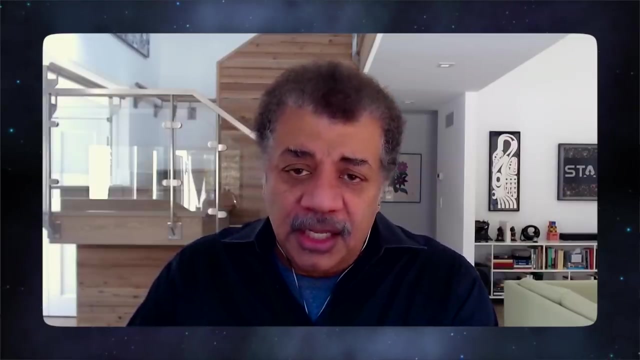 like that. i wonder what superhero would be made from omega rays. well, gamma rays are um. in the early days, before we fully understood what the sources of energy were, there were alpha particles, beta particles and gamma particles- alpha, beta, gamma and the alpha particle is a helium nucleus. 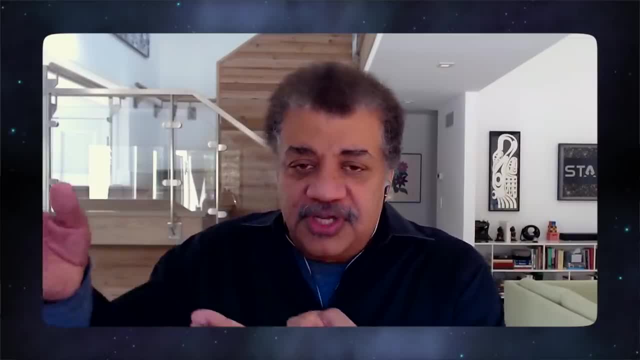 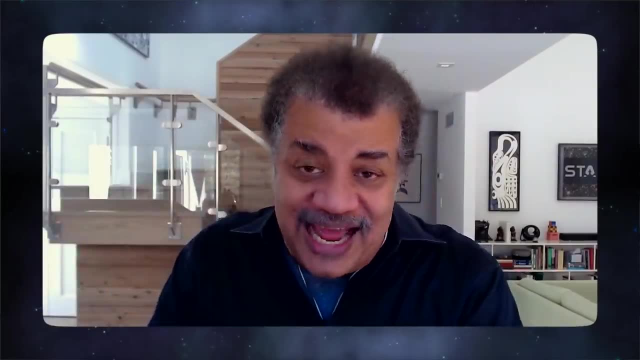 the beta particle is an electron and the gamma ray is a photon, but they all had energies that we could measure. so we're measuring the energies, not knowing what the thing was. the gamma ray caused it at the time, but that all splits out. so we have, um, like i said, ultraviolet x-rays, gamma. 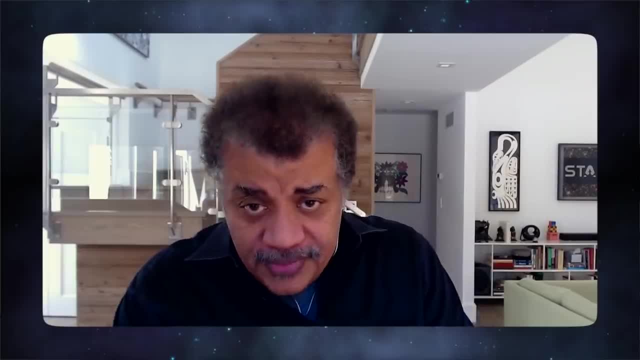 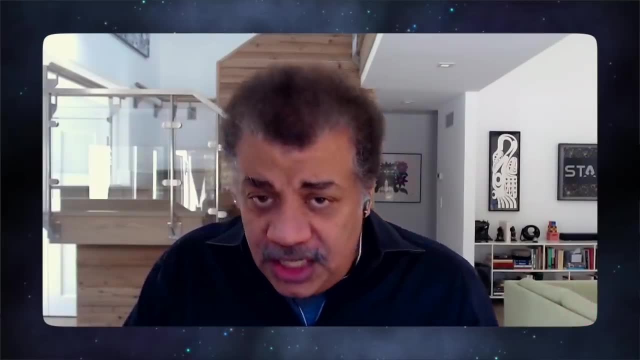 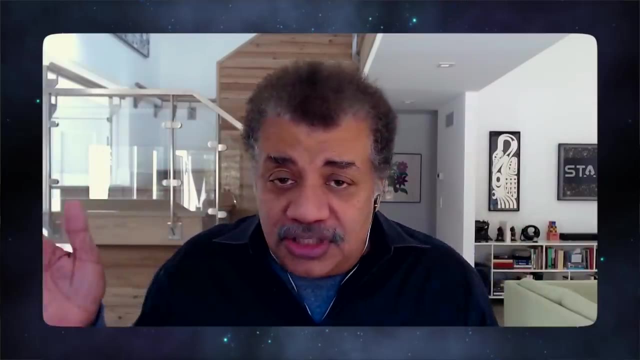 rays. there you have it all right. go the other direction. wavelengths are getting longer, the energy is dropping, so you go below the red. you get infra red below the red, all right. by the way, you can't see infrared. you can't see ultraviolet. if you buy, i want an ultraviolet bulb. we used to. 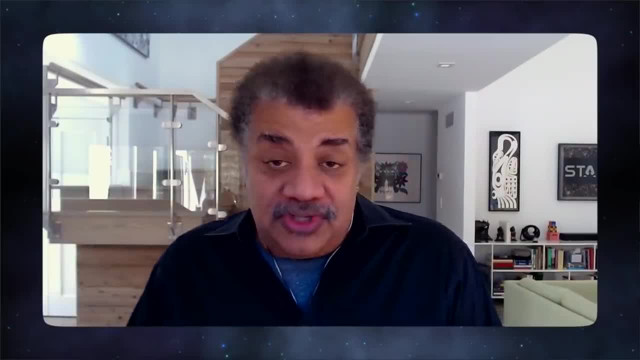 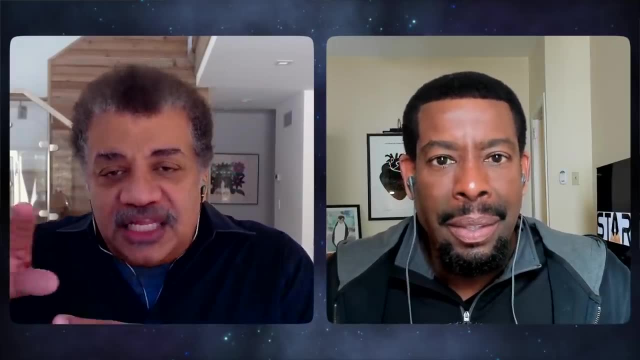 call them black light bulb. i want an ultraviolet bulb and you turn it on and you see it. you say i can see the ultraviolet. no, you're not. you're seeing the violet, right? okay, there's a little bit of violet spilling out. the actual ultraviolet you don't see at all. same with the infrared lamps. 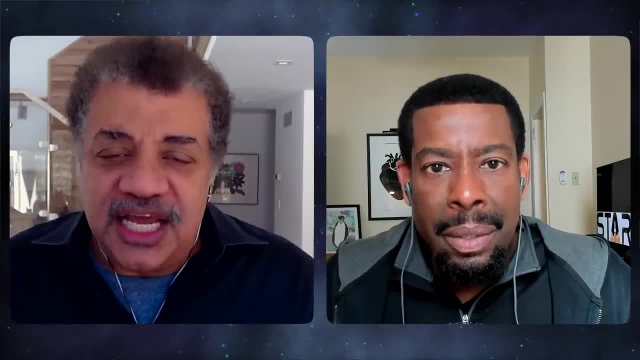 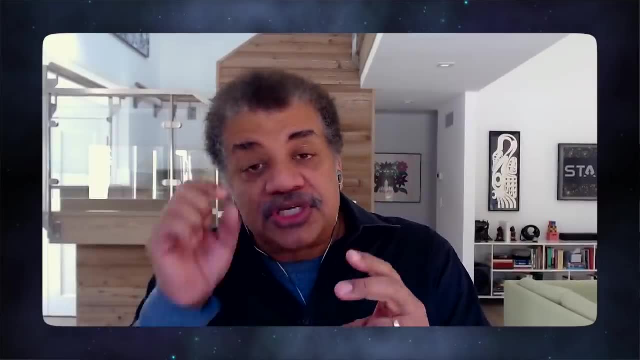 you buy an infrared lamp. if that was pure infrared, you turn it on. you wouldn't see a damn thing. okay, right, but a little predator, that's exactly so. a little bit spills into the red part, so you see the red emitted by the infrared lamp. all right, 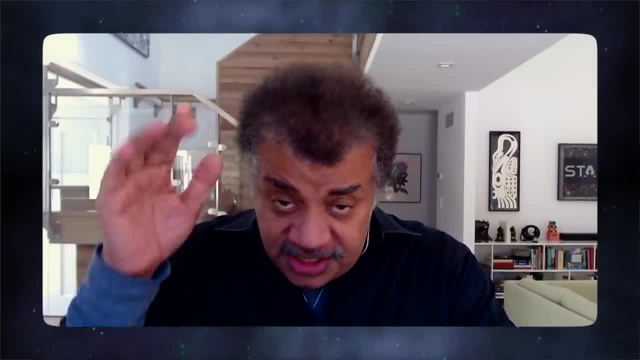 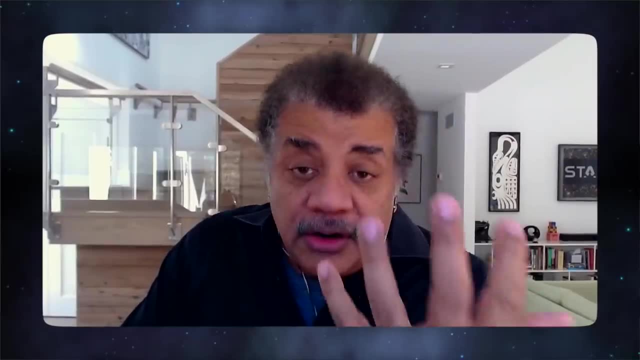 you're not a predator. we can detect infrared not by our eyes, but by our skin. you, you detect infrared as warmth, right, all right, it's a detector. think of it that way. all right, a warmth detector. so there's the infrared, and then you go beyond infrared. 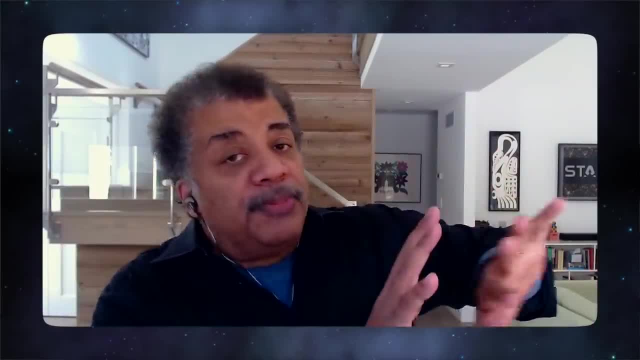 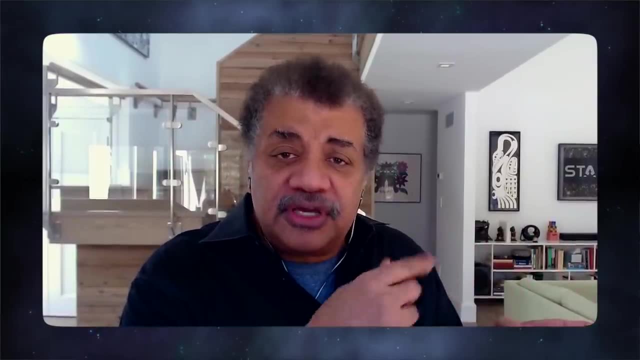 below infrared, the what used to just all be called radio waves. and then they said: well, there's a section of the radio waves that have special utility for us for communicating. it's just the shortest of the radio waves. and then they said: well, there's a section of the radio waves that 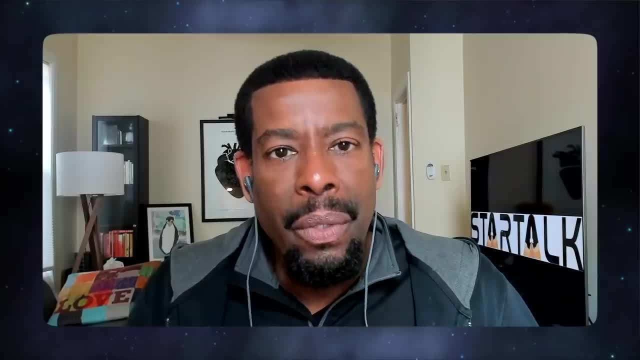 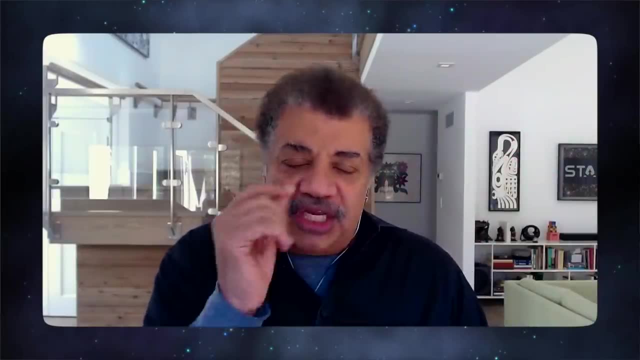 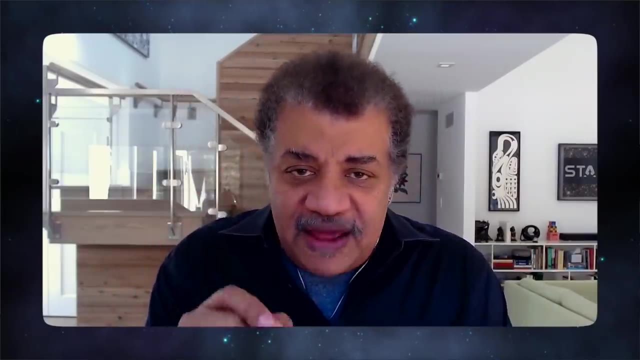 radio waves and they call them micro waves, sweet short radio waves, micro waves, so that that gets that got a labeled right there between infrared and radio waves and beyond microwaves we have radio waves, but and now we're getting physically realizably sized wavelengths of light. so 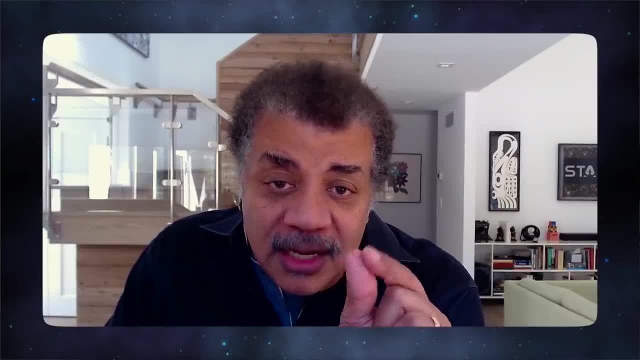 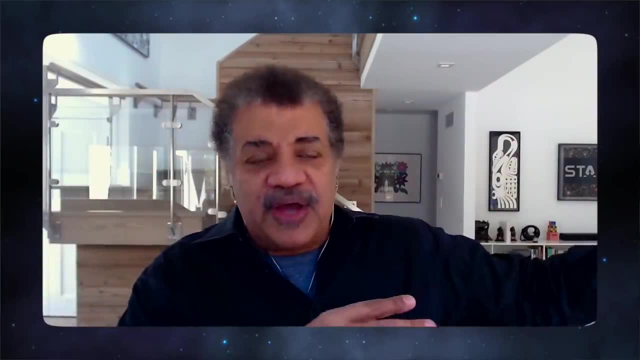 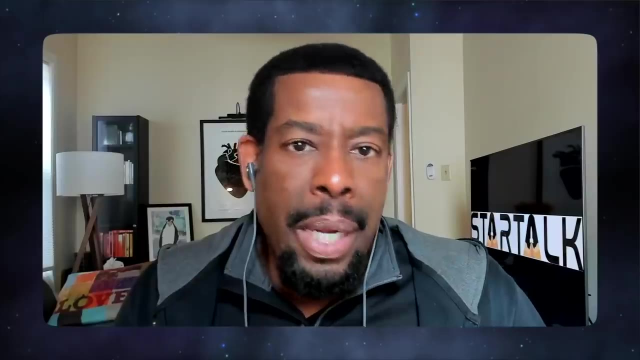 microwaves about a centimeter long. we can actually show that between a millimeter up through a few centimeters, and then we get into the meter zone, yards and things. those are radio waves and, once again, like like gamma rays, these just continue forever and we don't have more words for it, right? 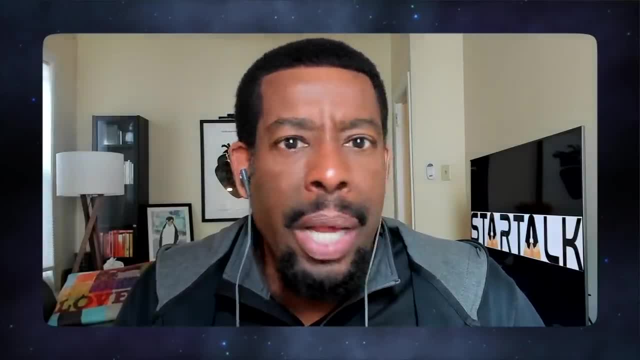 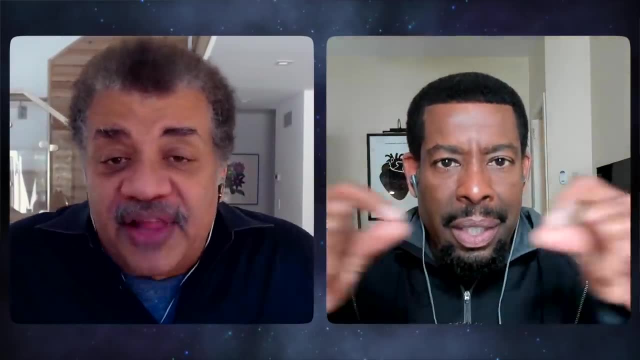 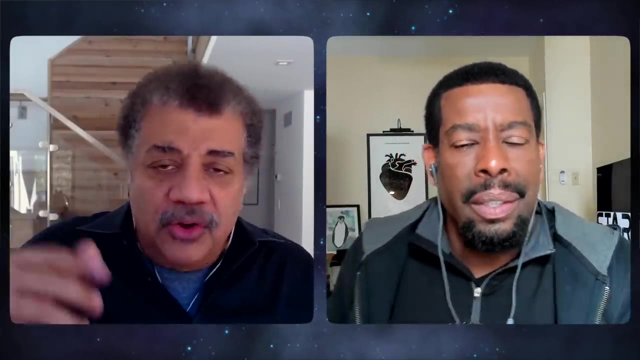 which is why we have so many different broadcasts, or is those just frequencies? but the frequency is the wave it you can call they, call it. call them wavelengths, right, but it's our habit to call them frequencies, right, right. so each frequency when you're tuning right on, in the old days you'd 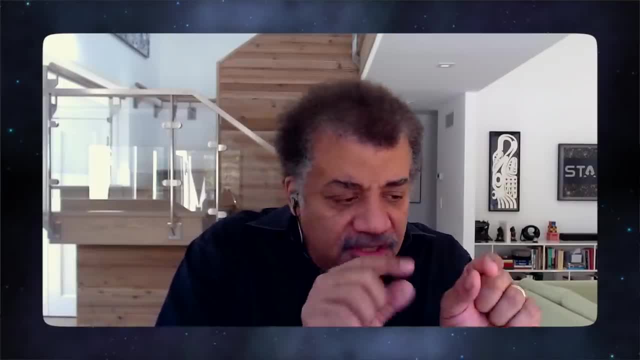 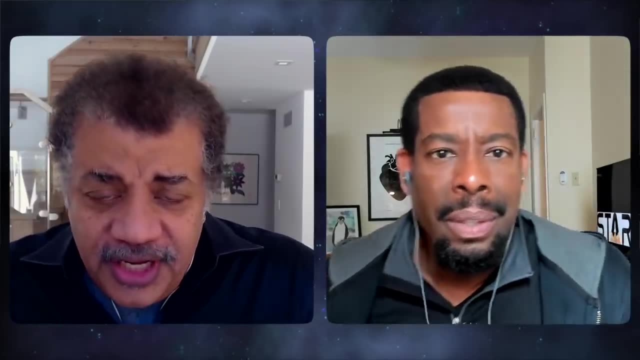 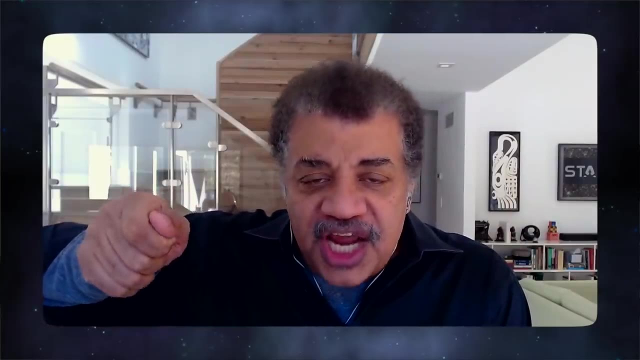 have an am or an fm radio, when you're turning the dial you are changing the frequency of your detector to receive a signal sent through that zone. wow, there you have it. that is, that's great. and in the old days, when you turn old timers, you turn the knob to change the channel on the tv. 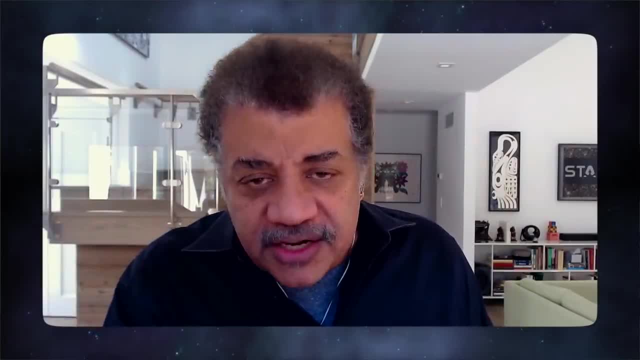 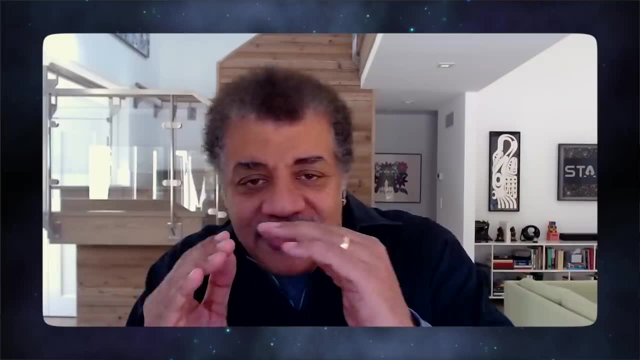 you're actually changing the frequency detector inside the television and there's that secondary knob that you could tune it a little sharper. i don't know if you knew that. okay, that that got you honed in on that one frequency. was it channel seven, channel eight? we just numbered them. 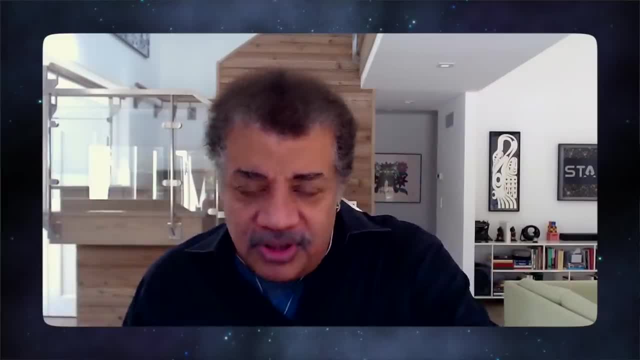 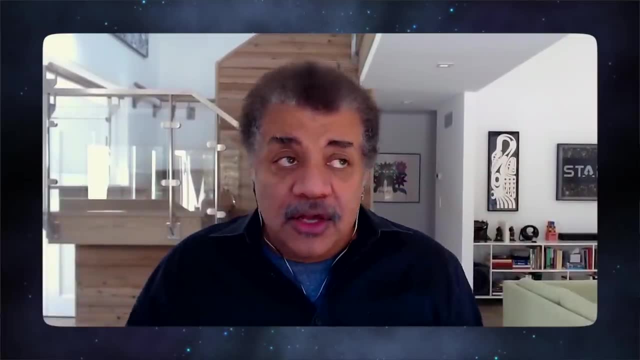 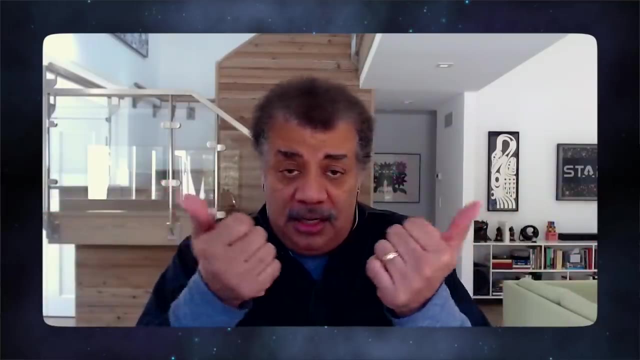 and we didn't give you the frequency because that's why, when you can just number them, which is what we did in the day, so anyway, all of these move at the speed of light. it is all light. most of it is invisible to you, in fact, if you put this on a scale, on a, on a, on a, if you drew all of these, 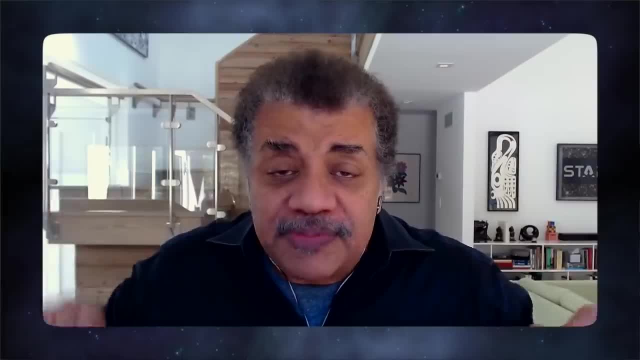 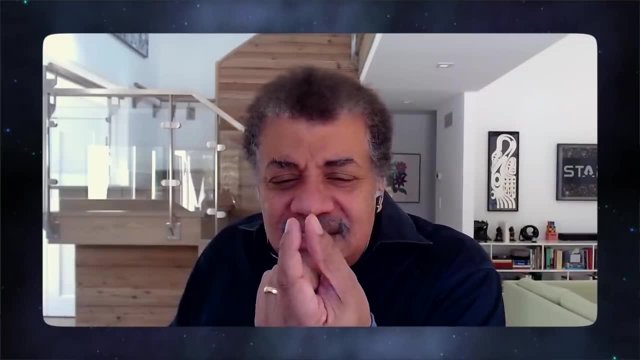 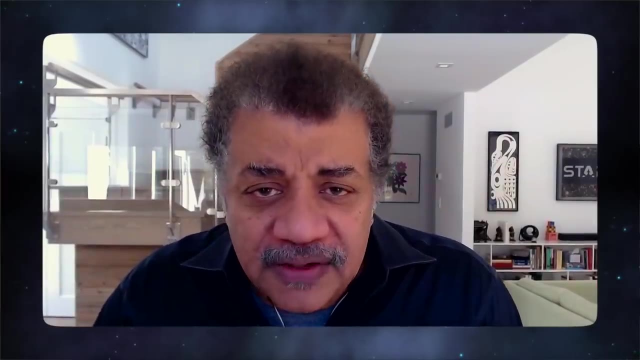 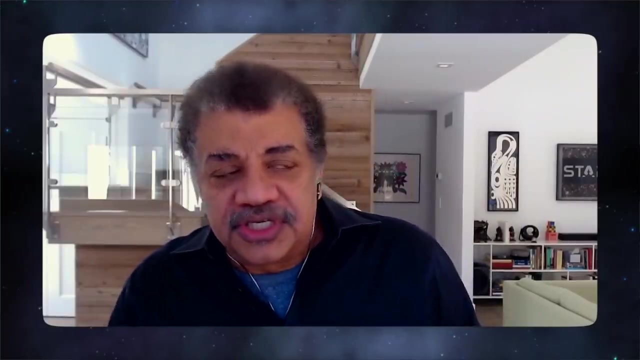 and you ask: well, how much of this whole electromagnetic spectrum can we see? right, and we see this tiny slice, this tiny slice among all these broad zones in the electromagnetic spectrum. we are practically blind. oh, and we didn't even know that until william herschel discovered infrared light. 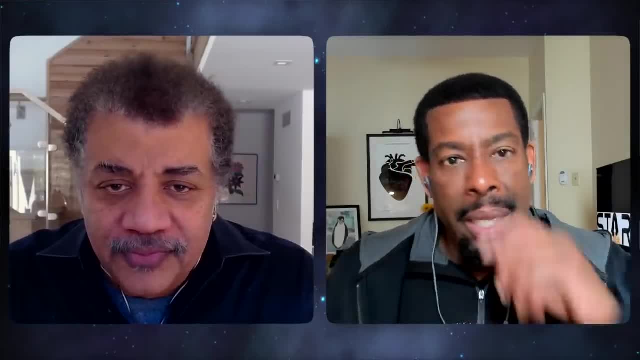 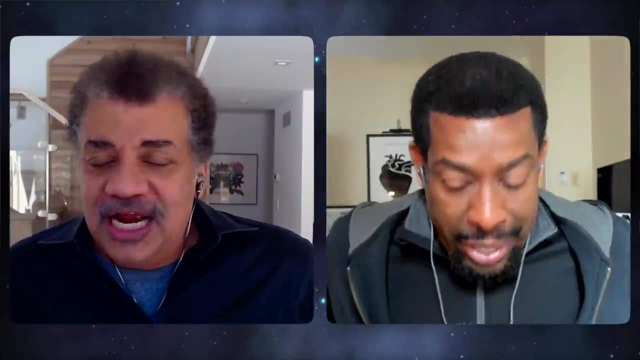 right, look at that. that is, and i think i said in another explainer how he discovered. i'll do it real quick now. you ready? i love this, i love this. yeah, i do remember. okay, herschel. herschel's a big fan of newton. newton has a spectrum, he shows the sunlight is composed of colors and you put a sort 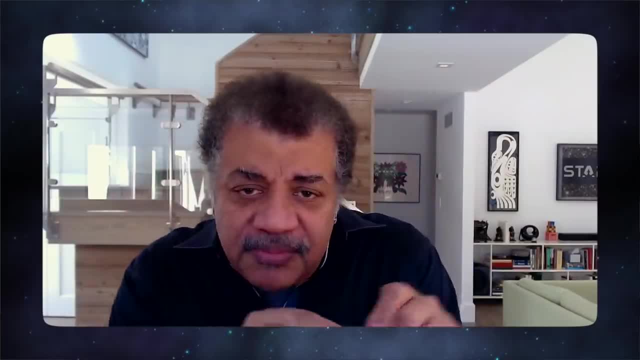 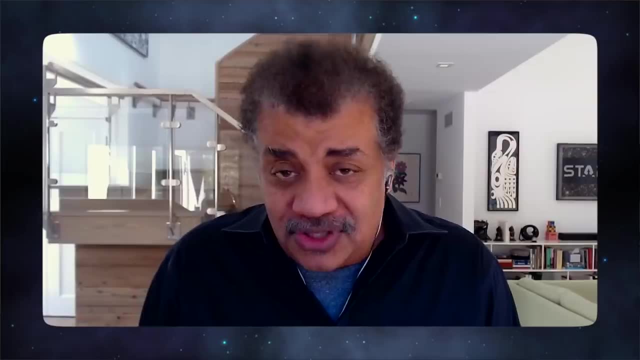 of slit in the curtains so the beam of light comes through your prism, so that it's dark elsewhere except where the prism light goes. and herschel said: i wonder what the temperatures are of each of these different colors. to even think, to ask that, yeah, all right, so he's got a thermometer. 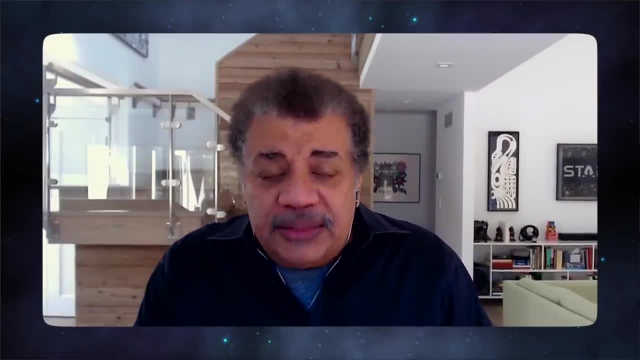 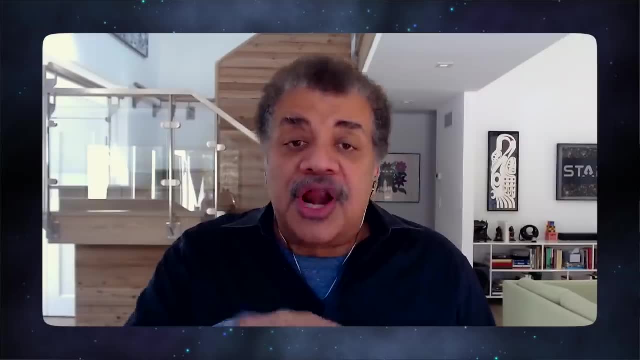 and he puts it in the blue and then he puts- and, by the way, it's an experiment, so you need a control thermometer- so you put the control thermometer- someone where, somewhere, where the colors are not all right- on the same table, but just put it outside the colors, which is what he did. 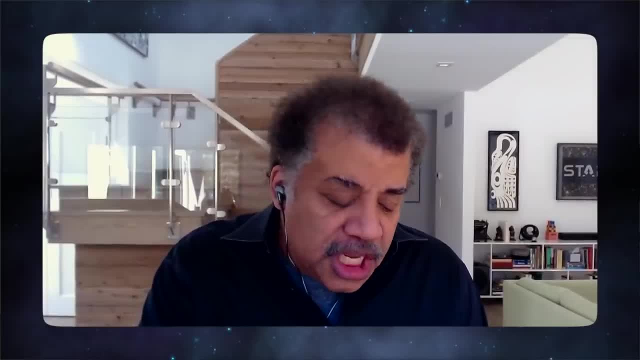 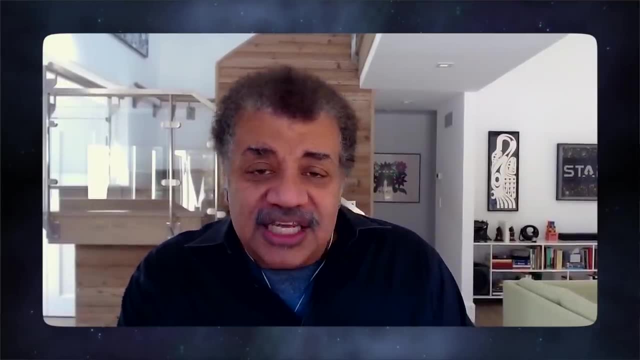 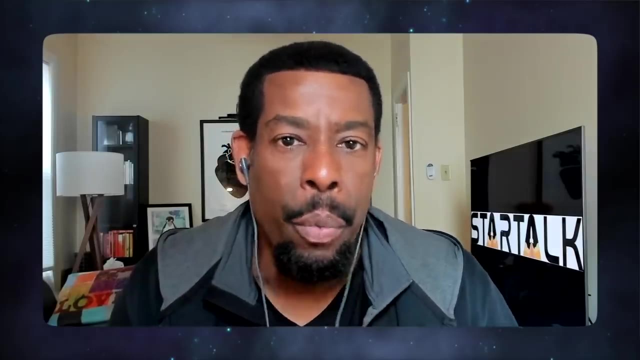 and he checked the temperature of the blue and the violet and the green and the orange and the red and he wrote out down all these temperatures and what he noticed is that the temperature sitting outside of the visible spectrum read the highest temperature of them all. right, and now why? 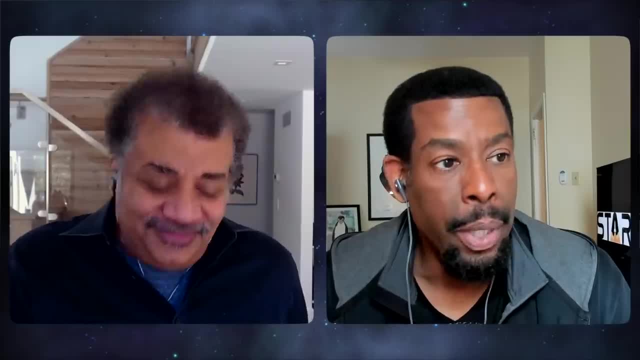 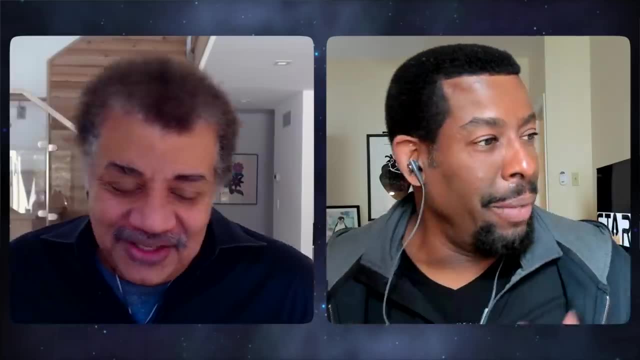 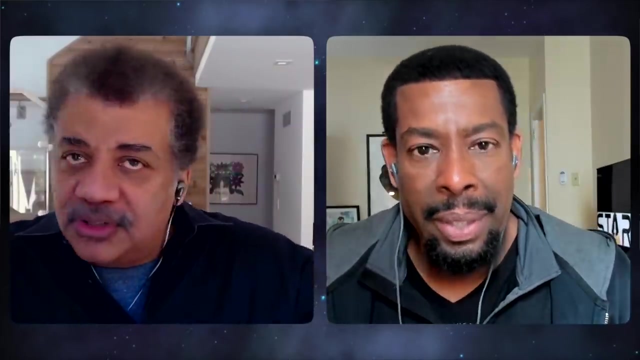 didn't he just say, oh, it must be hot in this room. i didn't realize how hot it wasn't here. maybe there's something wrong with me. i can't. i can't feel heat anymore. so so there it was. and because he didn't put the thermometer somewhere else, he 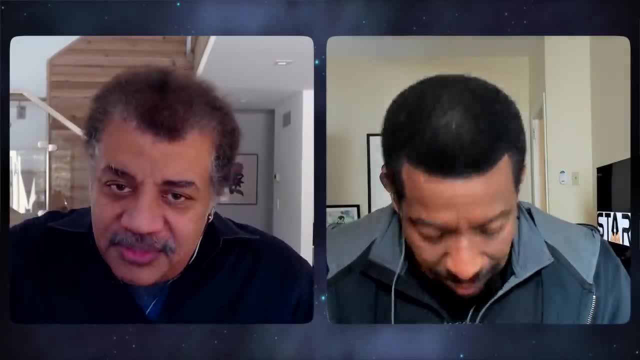 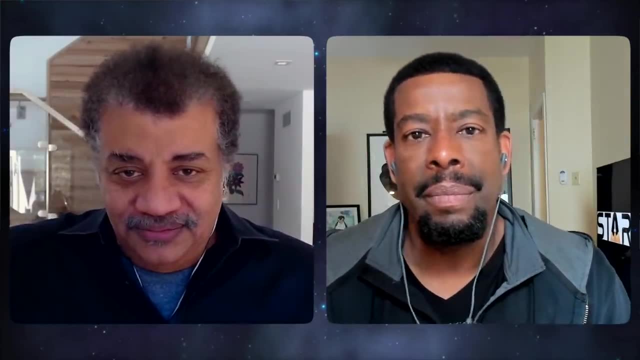 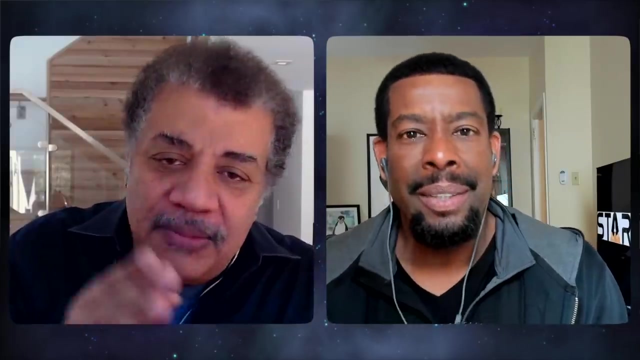 right next to it. right next to it because at the same environment as there. and he said, oh my gosh, there must be a form of light- quote- unfit for vision. that's a- i love the terminology unfit for vision, light and that's. And had that thermometer been on the other side of the violet, it's not clear that ultraviolet would have warmed the thermometer in this way. 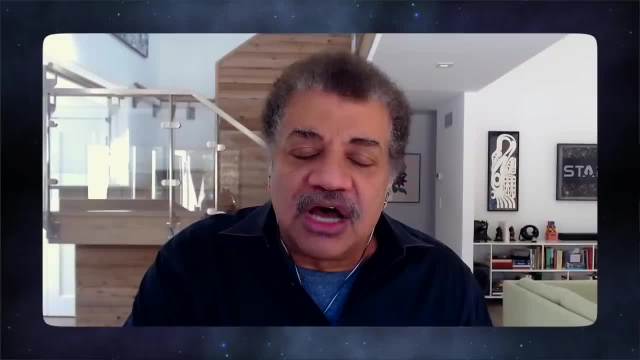 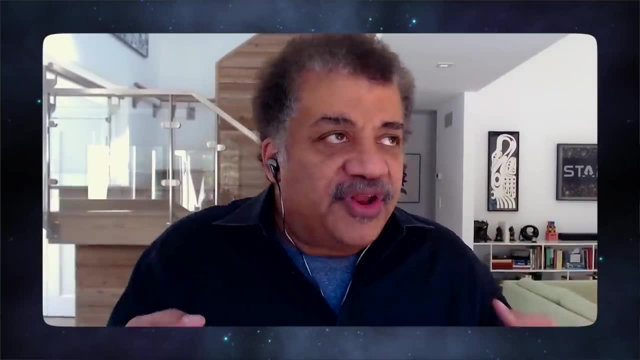 But he happened to have it on the side where the red was, and he discovered infrared light with that experiment. And so when I look at my microwave oven and I look at a radio transmitter, or I look at my cell phone and I look at my lamp on my table, 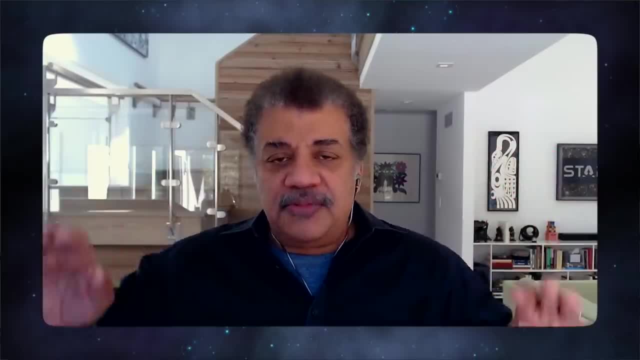 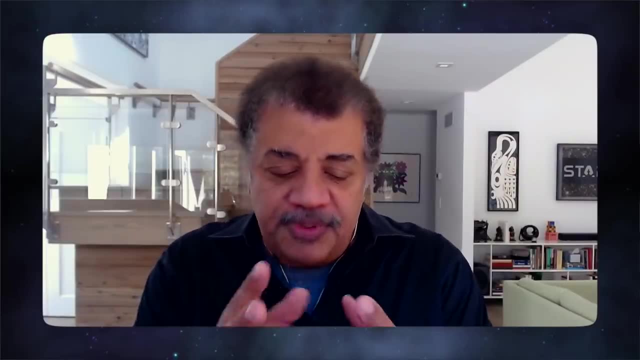 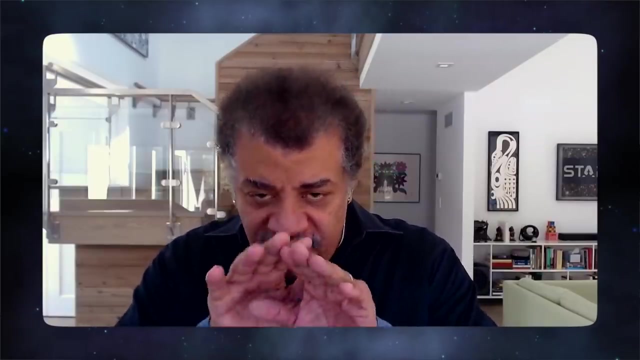 it is one happy family of electromagnetic spectrum coming to us. That's so cool. It's dope And it's called electromagnetic because it's a wave that simultaneously moves between being an electrical wave and a magnetic wave, and it's self-propagating through space. 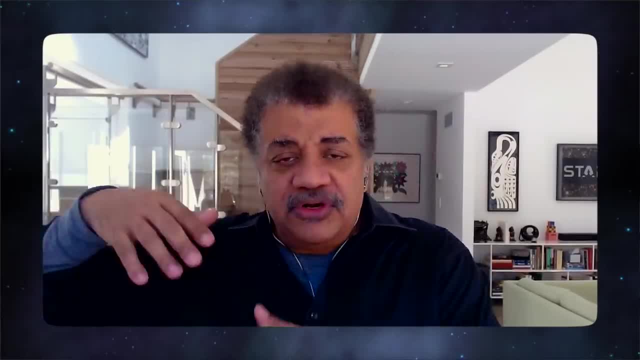 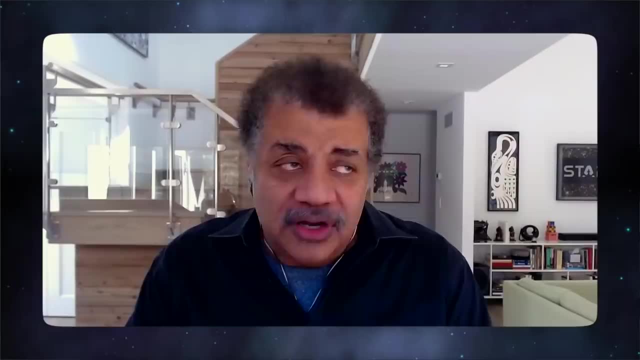 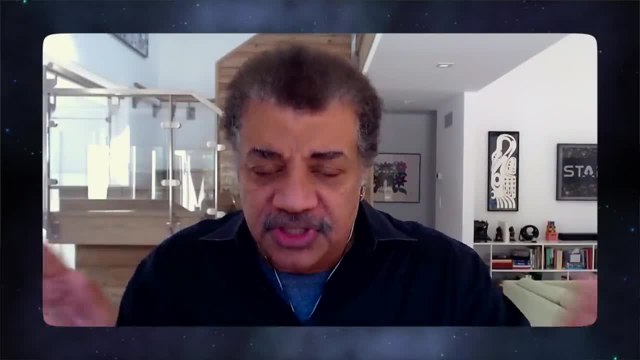 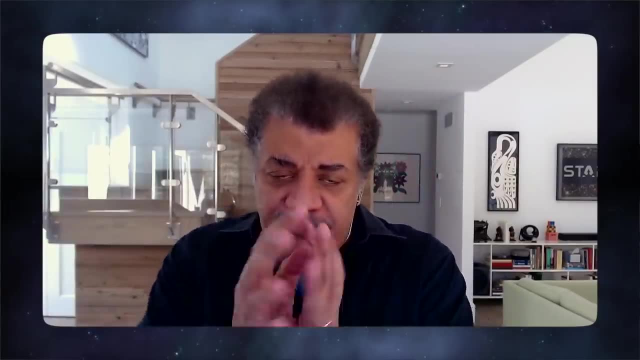 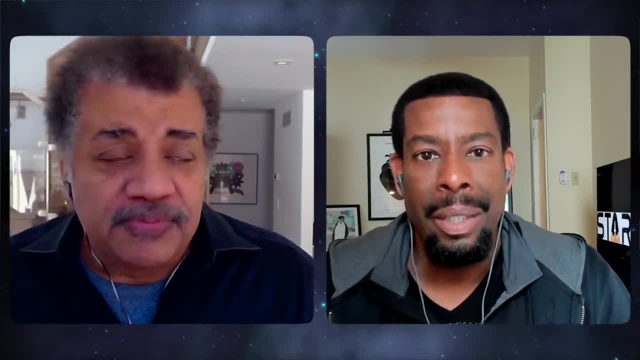 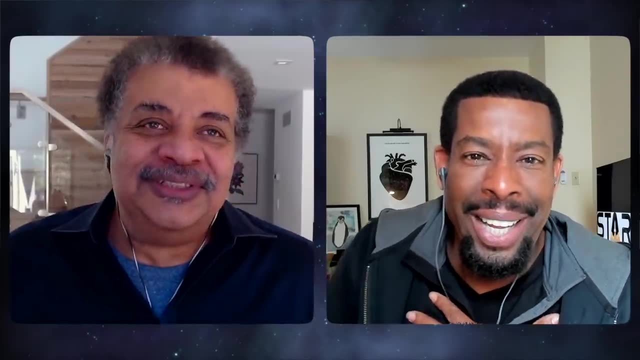 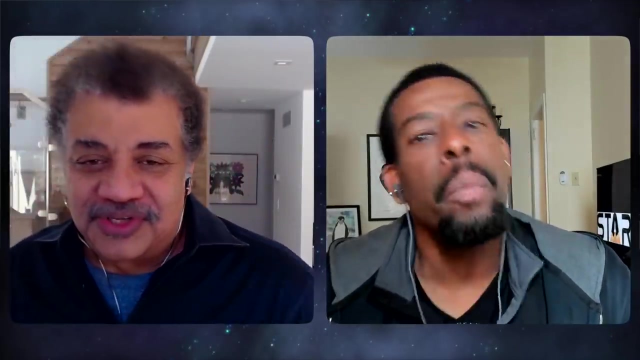 There you have it, Chuck. That's great. And it all started with my potatoes Just saying: And what wavelength are they on? The delicious wave, The delicious, The delicious. We keep them warm with infrared. It all comes full circle. 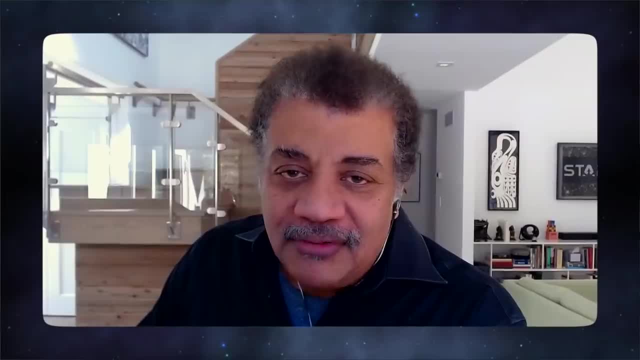 That's so true. All right, Chuck. that's all the time we got. All right, That was great. All right, That's been another explainer from StarTalk, Neil deGrasse Tyson, here. Keep looking up.